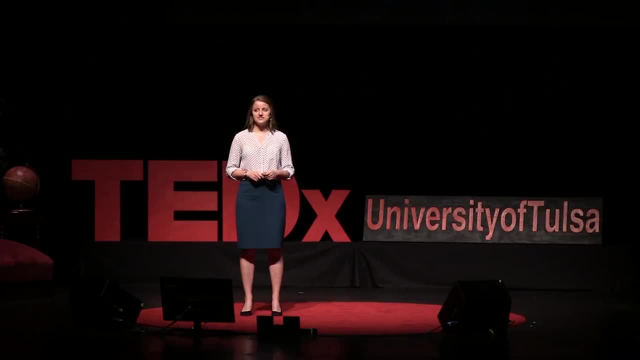 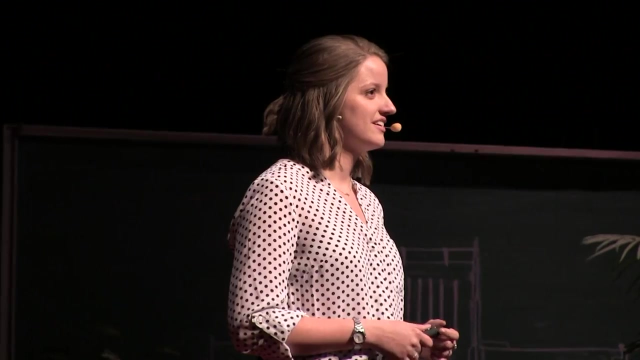 we're told about the spaces where we live. cities have never been able to completely mask the problems that almost all of them have in common: Poverty, inequality, vacancy, unemployment. these things follow us everywhere. I dare you to find a city in the United States. 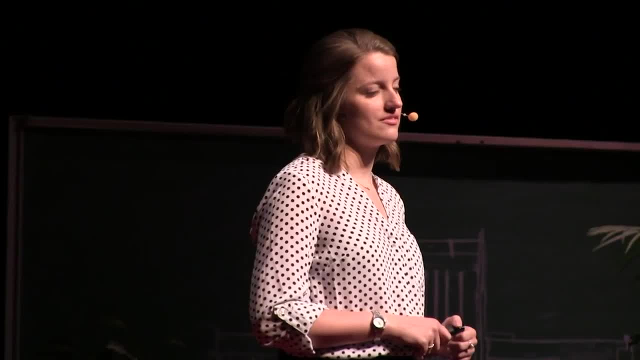 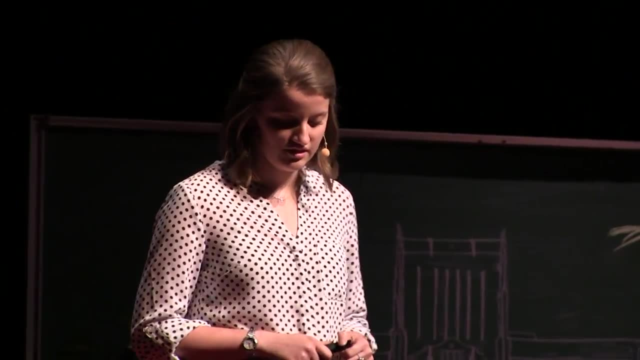 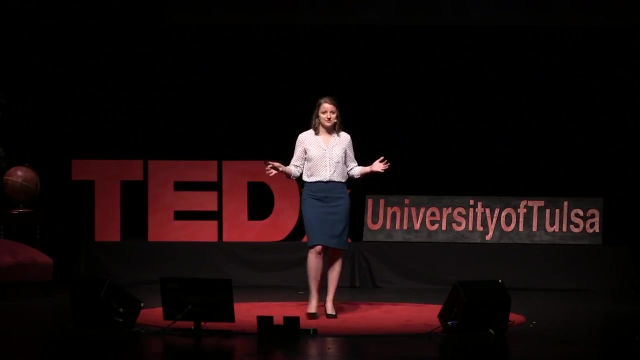 that doesn't struggle with any of these things. They're very hard to escape in this country, And in some places they've caused irreparable damage. Could public transportation be the answer? Now, bear with me here, because I'm not suggesting that we all give up our cars and start riding buses everywhere. I'm not ready to do that. 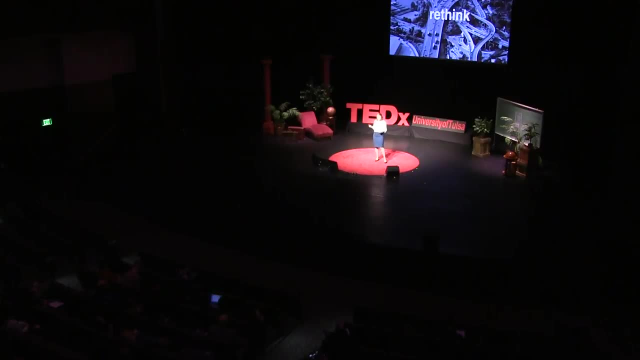 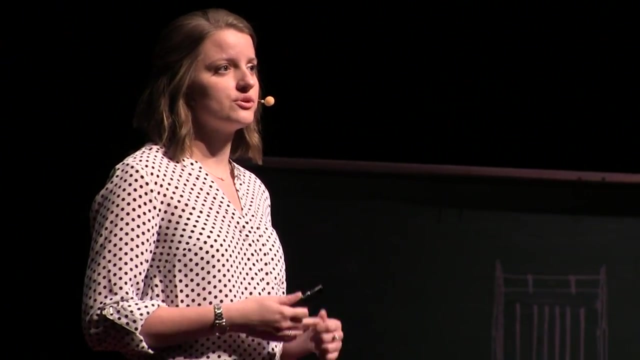 yet either, But I believe that rethinking our roads could help us to solve some of these problems, Because, think about it, Roads are everywhere and everyone uses them, regardless of if you have a car or a bike, or even a home. Roads are so central to our lives And we. 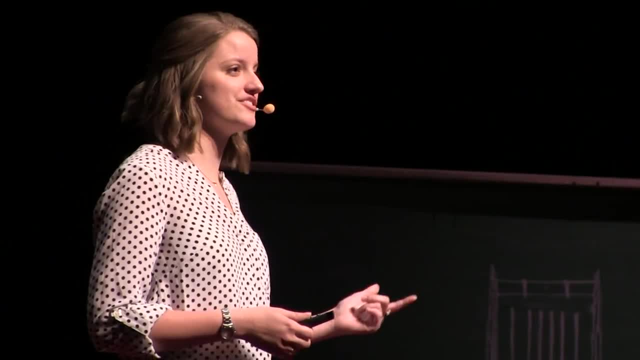 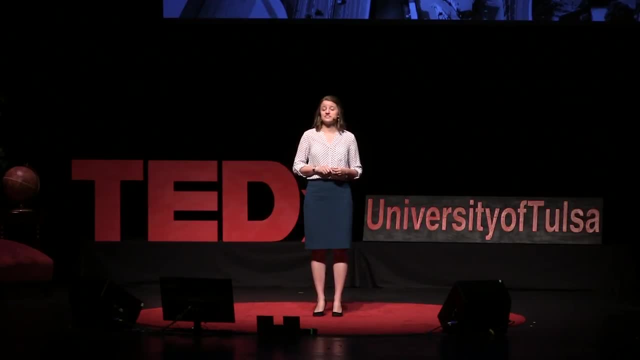 are so central to everything that we do, But are we using them to their fullest potential? Solving these types of social problems can be challenging because we're dealing with the ultimate variable: humans. The famous astrophysicist Neil deGrasse Tyson once said: 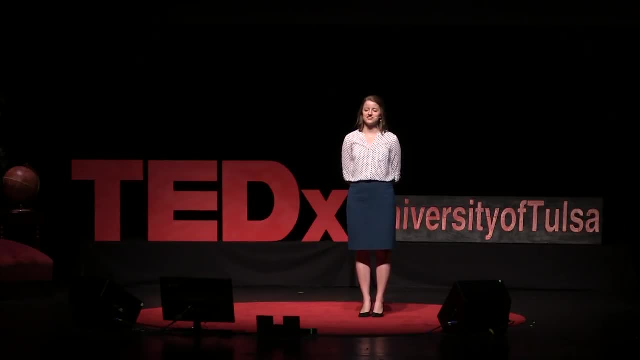 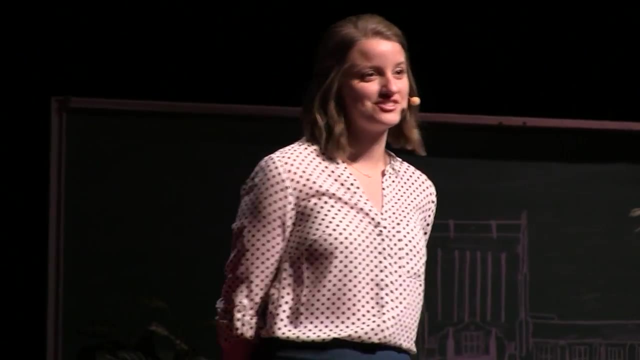 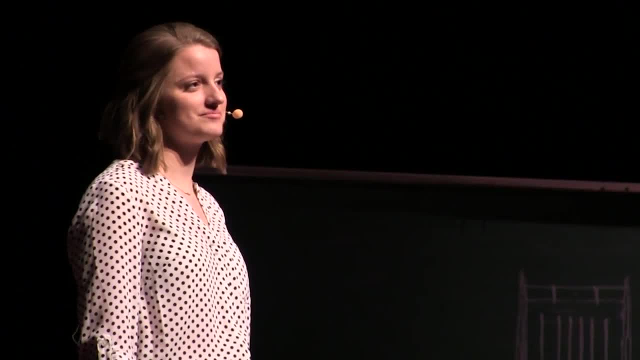 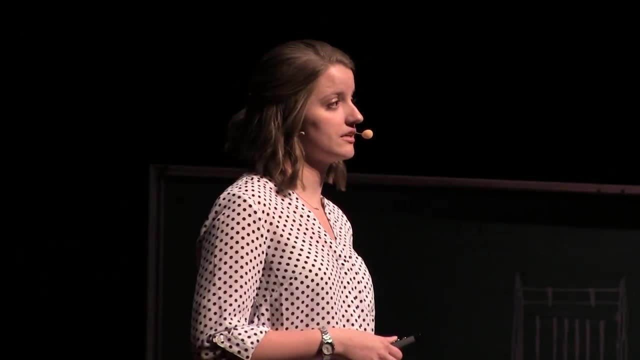 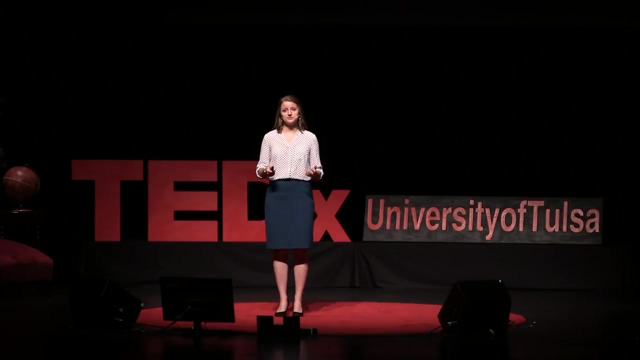 simple. It's just that humans are complicated. Things like physics and chemistry are the same everywhere in the world, But sociology and city planning take different forms in different places. because they deal with humans. And because we're dealing with humans, research also gets a little complicated. We can't really generalize the solutions that work for one. 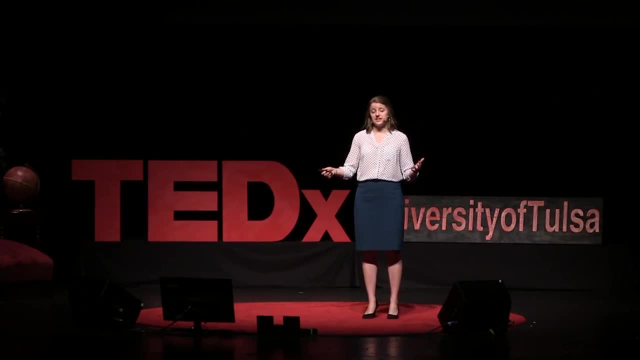 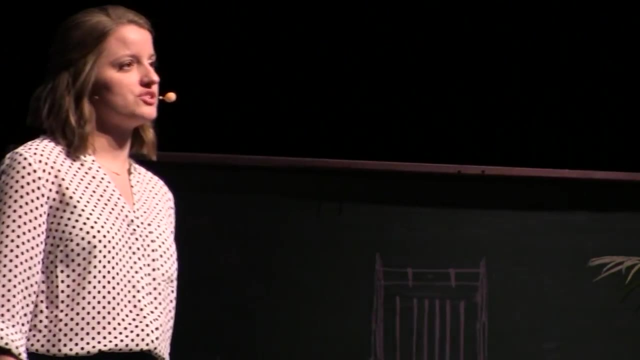 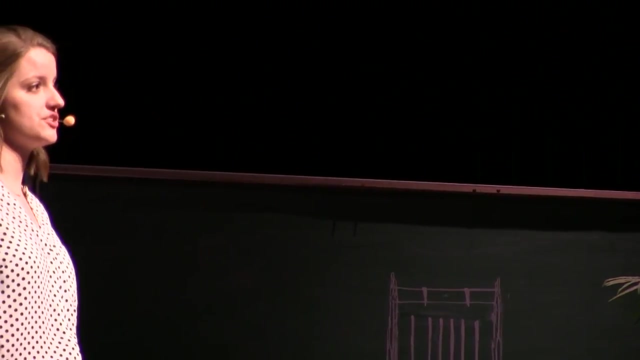 area to an entire country, So researchers tend to conduct research in different areas. Researchers tend to conduct research. City planners tend to conduct research using case studies. I conducted one such case study which focuses on Dayton, Ohio. Now Dayton has experienced massive population loss. over the last 50, 60 years It has lost almost half of its people. 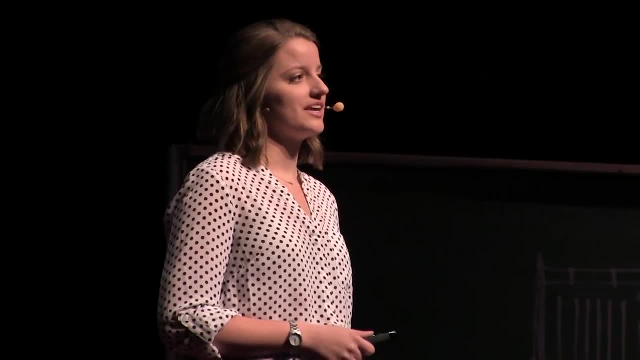 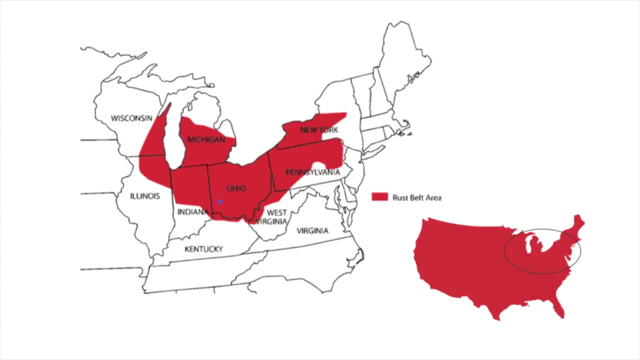 primarily as a result of deindustrialization. It's located in a region famously known as the Rust Belt, And in this region, during the mid-1900s, the manufacturing industry moved south very rapidly, So this was once the manufacturing and production hub of the. entire country In the mid-1900s. that all changed. The industry moved south, where production was cheaper, Factories and equipment were left abandoned and many, many people were out of a job. So this has resulted in massive inequality and a huge amount of decline In. 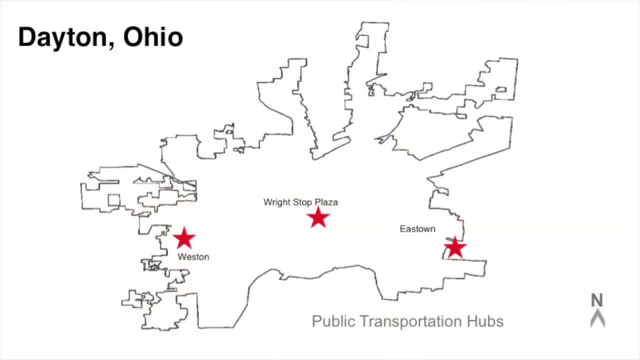 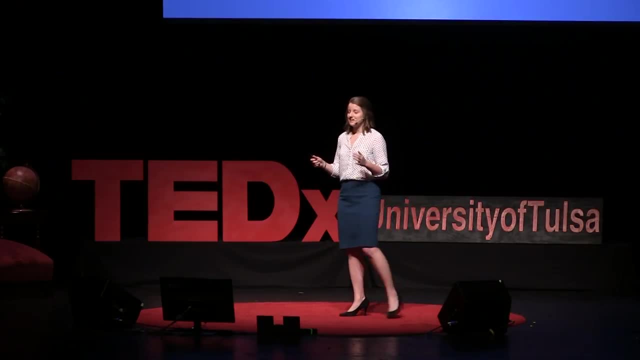 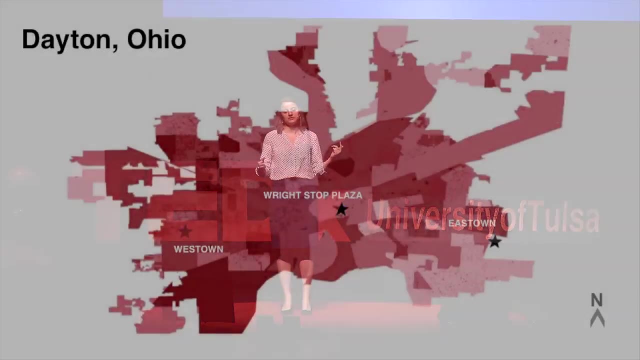 the city of Dayton. there are three large bus stations that serve as major transportation hubs for the city. What I did was create a decline index that essentially measures the decline in the city, a big composite variable. On this map, the darker spaces represent more. 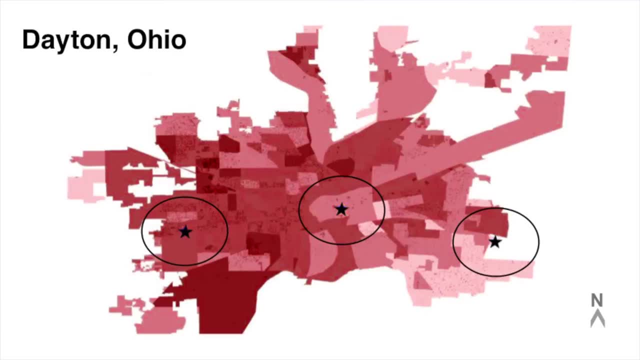 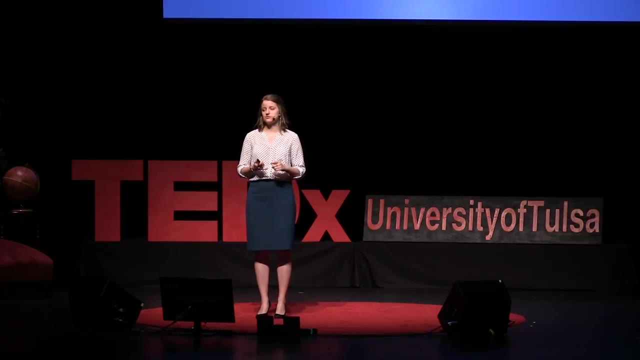 severe decline and the lighter spaces more stability. What I found after comparing the space around each of these hubs to the space in the rest of the city was that greater access to one of these hubs was correlated with greater stability. So that's the social problems that I mentioned earlier: Poverty, unemployment, plus things. like vacancy, unpaid taxes, structurally unsound buildings, delinquency- All of these things decreased the closer we get to a bus station And within one mile of a hub there was not actually any severe decline at all. The reason I chose one mile to analyse is because this: 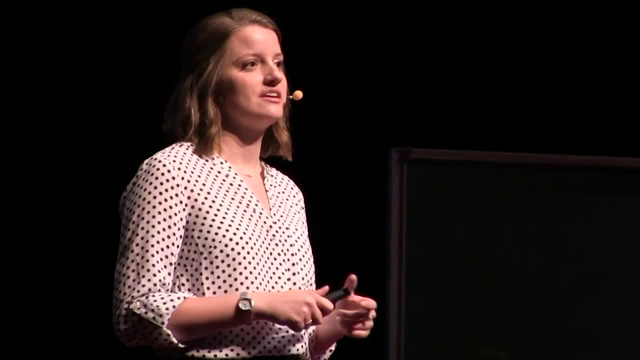 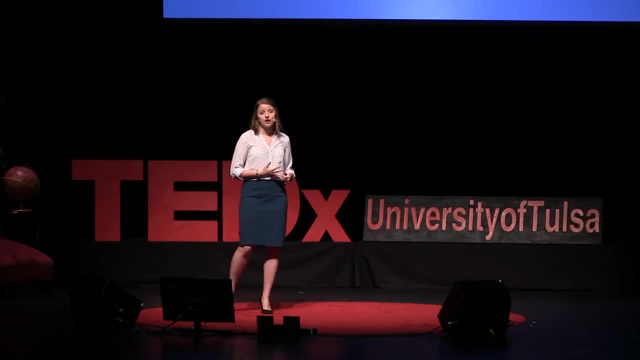 is kind of like an accessibility threshold. That's one way to think about it. That's the of it. Past a mile, this resource becomes much less accessible to people. So if I don't have a bike or a car or another quick way to get around a city and I 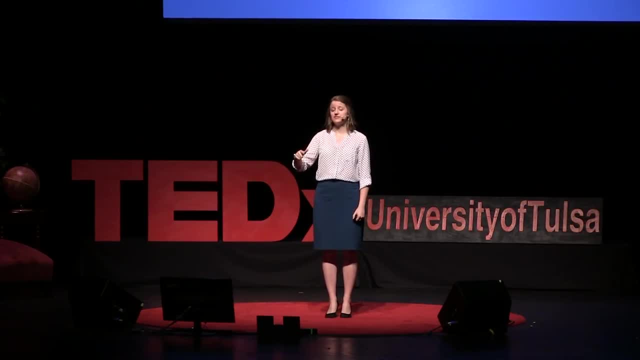 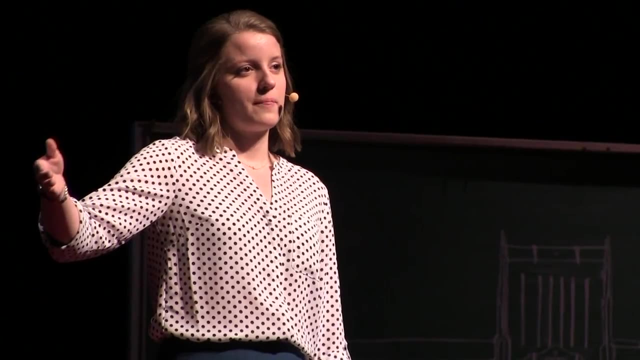 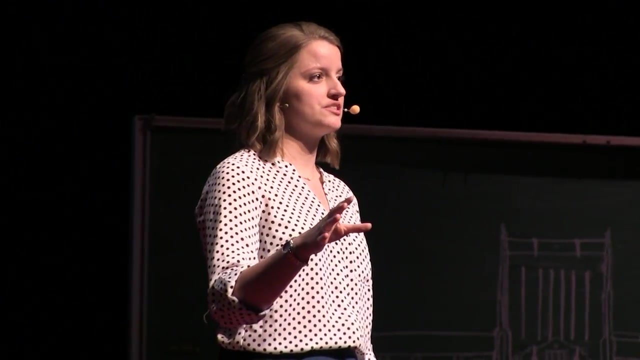 live more than a mile away from a bus station, the accessibility of that resource to me decreases drastically because I have further to walk before I can reach it right. One mile is kind of like walking from the White House in Washington DC to the Washington National Monument, Or to break it down more. 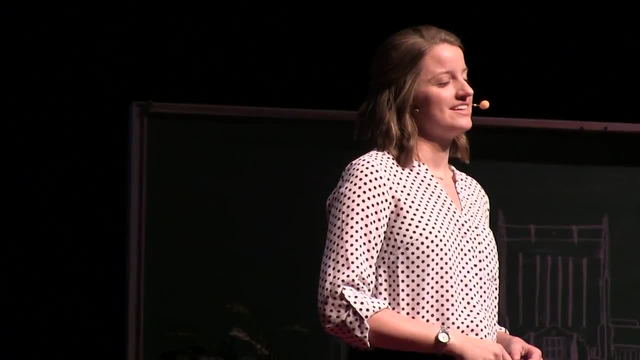 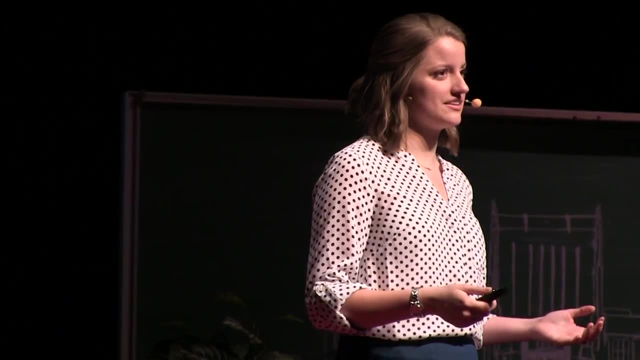 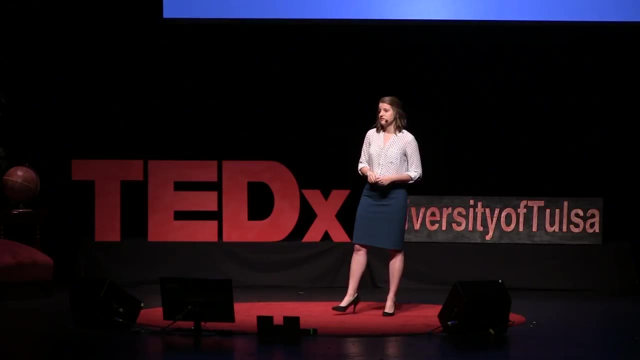 locally. one mile is like walking from the University of Tulsa campus to the Reeser's grocery store on 15th and Lewis just to catch a bus. All of a sudden, that public good becomes a little less good for the entire public. Similar research. 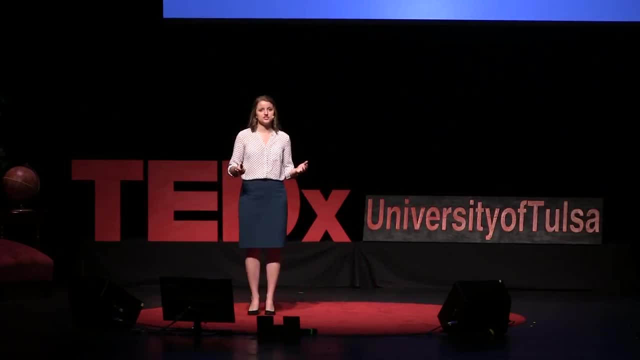 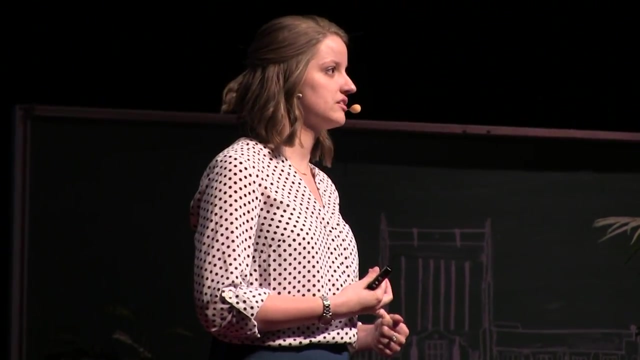 out of Portland State University suggests that better access to transportation can help to improve health outcomes for people in low-income neighborhoods, and many urban research institutions support this idea that greater access to transportation can help to alleviate poverty, decrease inequality, help to recover people who are considered vulnerable socially or